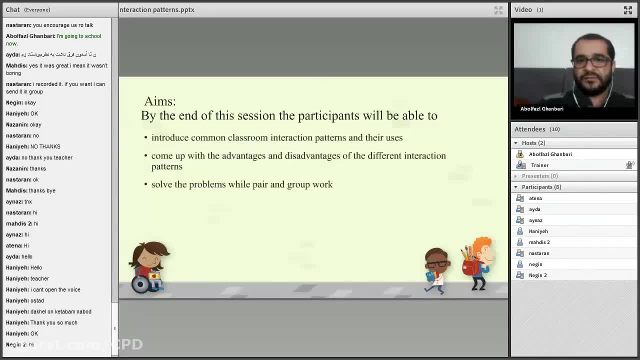 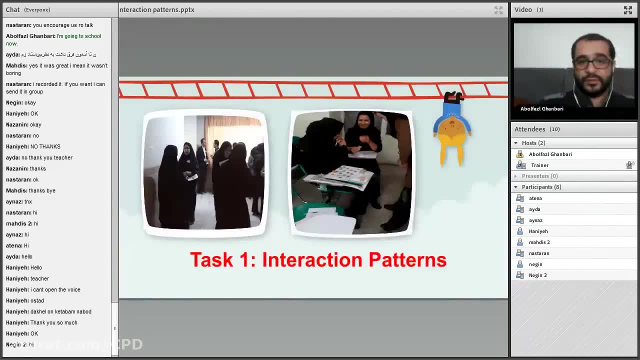 Come up with the advantages and disadvantages of different interaction patterns and solve the problems while pair work and group work. So here you see, two types of interaction patterns. Can you say the name of these two types of interaction patterns? What are they? Do you know? 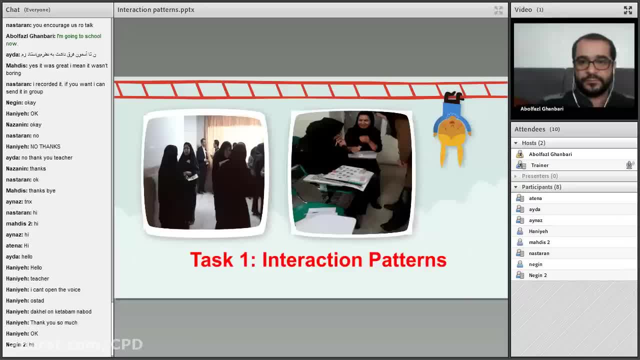 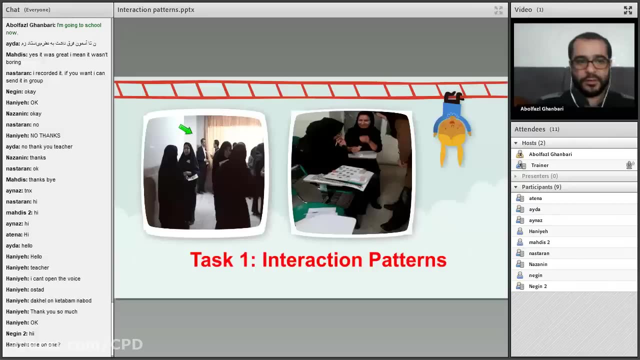 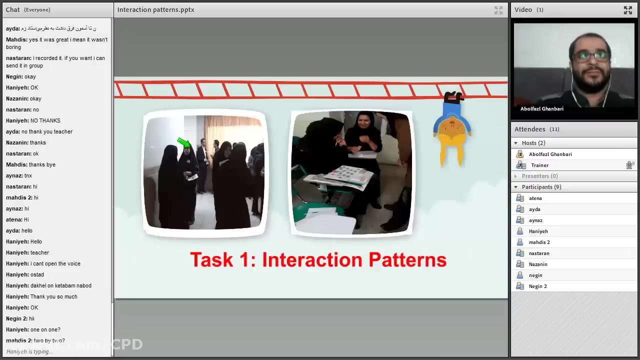 What is this type of interaction pattern? What do we call it? It is one, two, three- They are three- working with each other. We call it group work- Yeah, Group work, activity, Group work. What about this one? The students walking in the classroom and when they meet each other, they start speaking. We call it mingling Mingle- Yeah, Mingle. 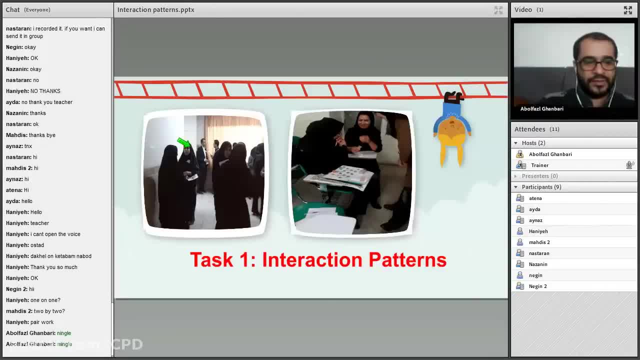 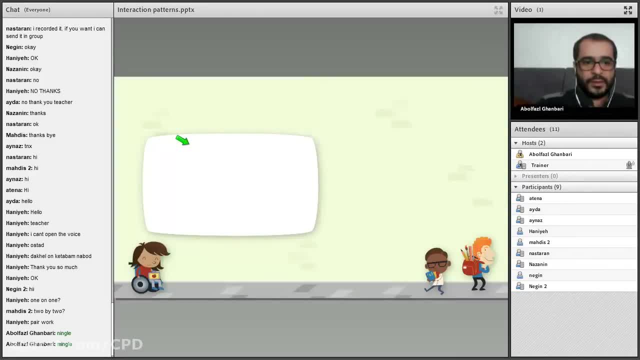 We just call it mingling, we just call it a tipo de utilización, Hop. So look at this picture. Can you guess what is the name of this type of interaction pattern? They, students, are working together. What do you call it? 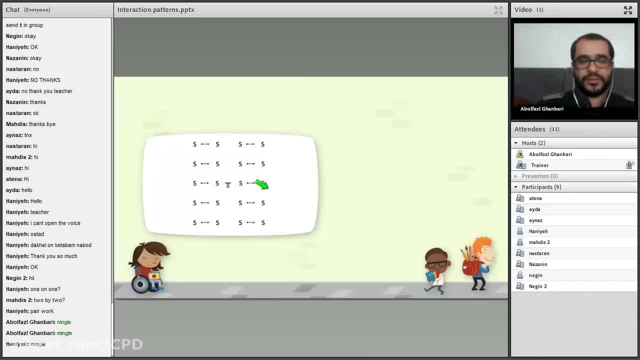 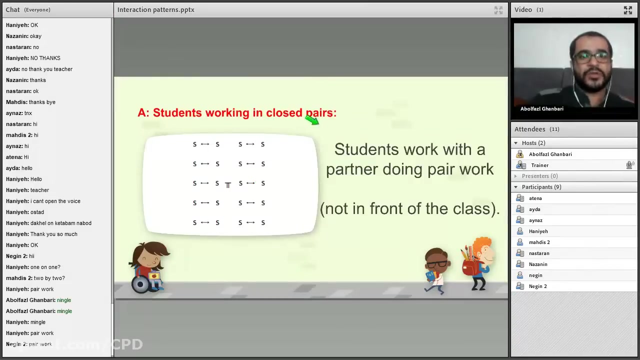 What do we call it? This is not mingling. The students are sitting in their chair, sitting in their seats and working pair. It is pair work. We call it pair work. Exactly, We have two types of pairs: Open pairs and closed pairs, Open pairs and closed pairs. Here we have closed pairs. In closed pairs, students are sitting in their seats, They are not in front of the class. We call it closed pairs. 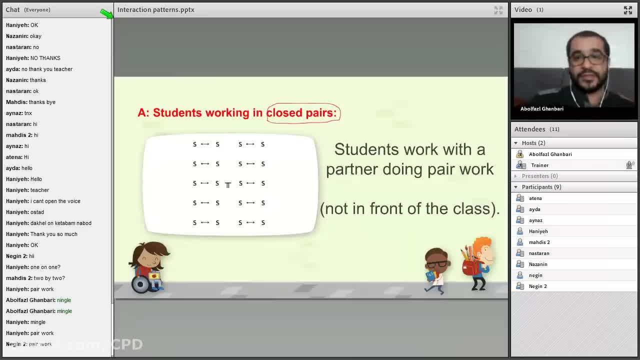 And all the students work in pairs And all the students work in pairs simultaneously at the same time. Can you say what is the advantage or what are the advantages of this type of interaction pattern and what are the disadvantages? Can you say Microphone will sound good, It looks fine Microphone, you hear. 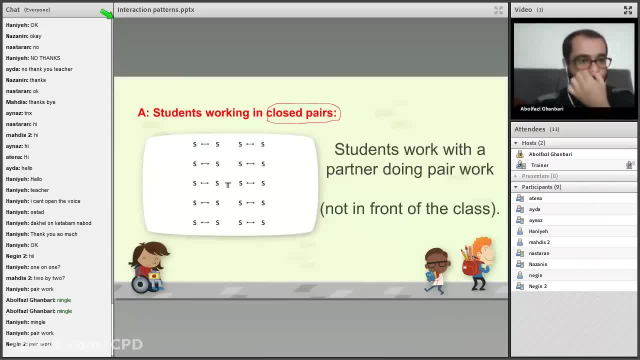 One advantage at the end, Say one advantage of pair works. May I Yes? or why not Turn on your microphone and start? I am waiting to hear you. I am waiting to hear you. Excuse me, my phone got off. Okay, I think that disadvantages may be their self-confidence to not grow to speak English, because when they are pair working students. 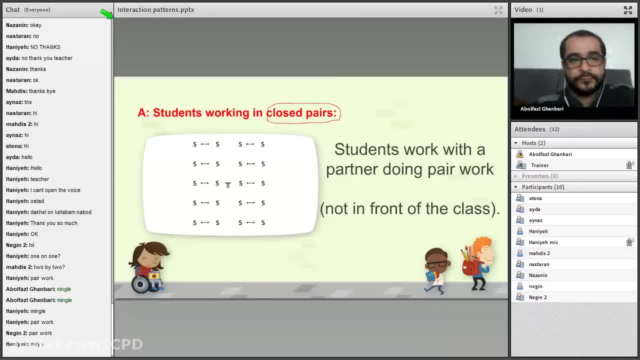 and they are not in front of the class. Excuse me, sorry, I have a problem here. You mean that when they are not in front of the class they may lose their confidence? No, I mean when they make a mistake, they are afraid to make mistakes in front of the class. 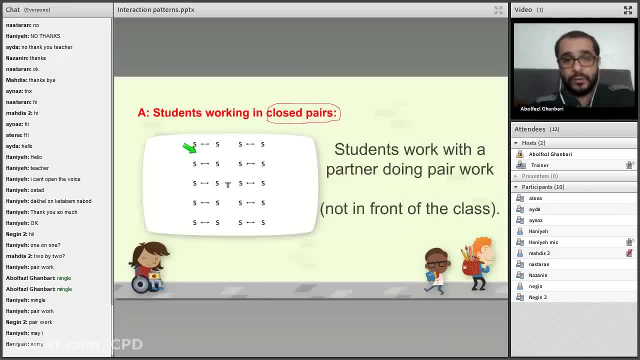 You mean that when they are not in front of the class, they may lose their confidence? No, they are not in front of other students. They are in front of their partners, just their partners. They are in pair. They are not in front of the class. When you ask them to come in front of the class, they may lose their confidence because of their mistakes, as you said. 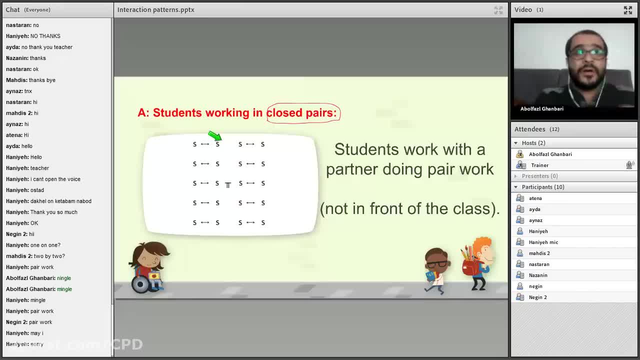 But not in pair. When you are talking just with your partner, just with your partner and other students are working with their own partners, you are increasing your confidence. You are feeling You start communication easily, Without any stress, without any punishment. 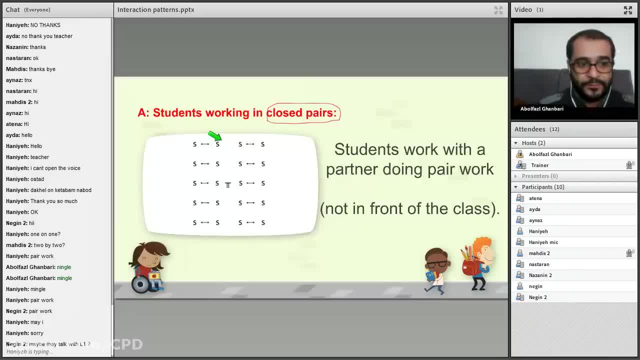 You talk easily. Yea, You talk easily. So I see the disadvantage is they have less information against the group work When you work in a group. they have less information against the group work. When we work in a group, we have a lot of information of different people and students. 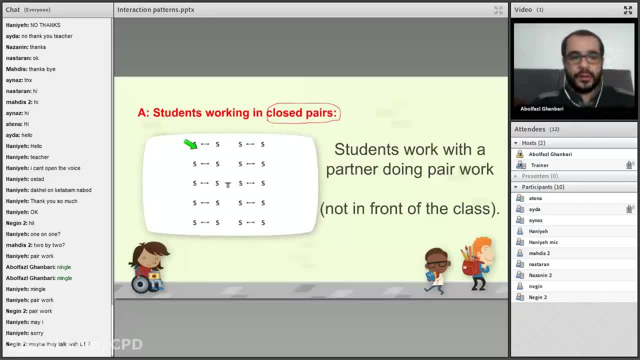 but when we work in paid work, Yeah, exactly exactly. They may have less information rather than the group work And because of that, the students may not talk, may not communicate, may not interact, because of the lack of knowledge they have, lack of information they have. 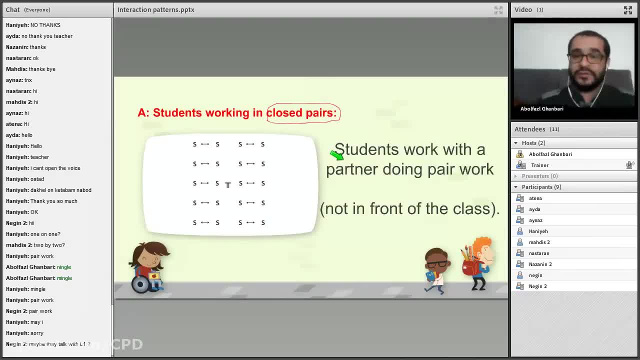 They stop talking with each other. It is one of the things we said. For another example of advantages, we can say: increasing our communication. For example, we share our ideas together and learn how to share our ideas. Yeah, by using close pairs. 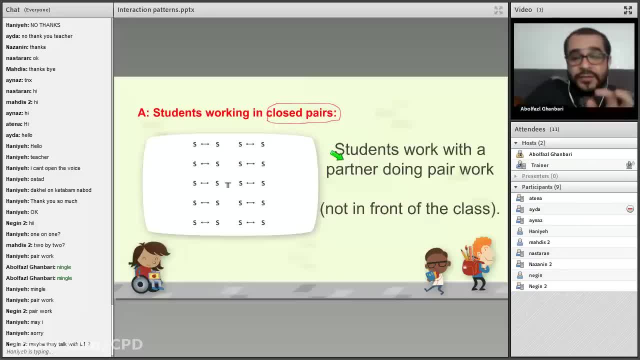 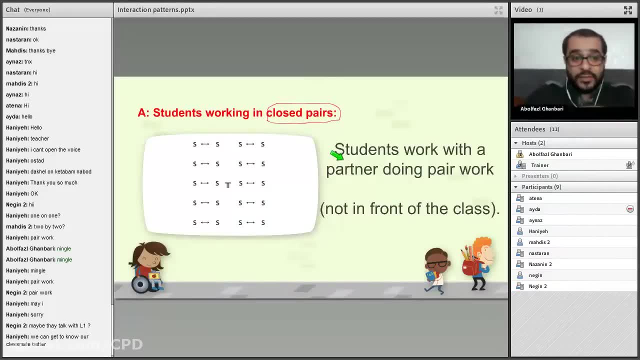 you can give the students opportunity to talk with each other at the same time. At the same time, all the students talk with each other, all the students. I guess you ask just two students to talk. two students And other students be silent. 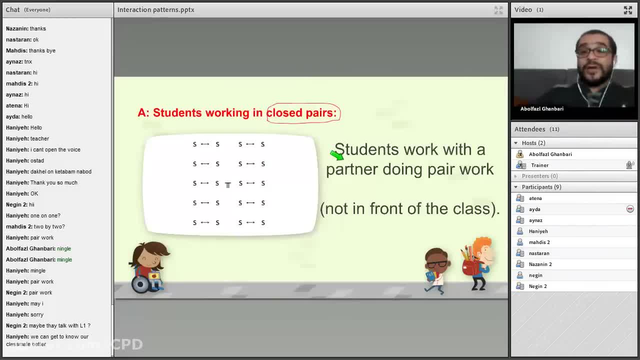 They don't have the opportunity for talking. But when you ask them to talk at the same time, to work in pay at the same time, they don't have the opportunity for talking. If you have five minutes, yes, All the students use this five minutes for talking. 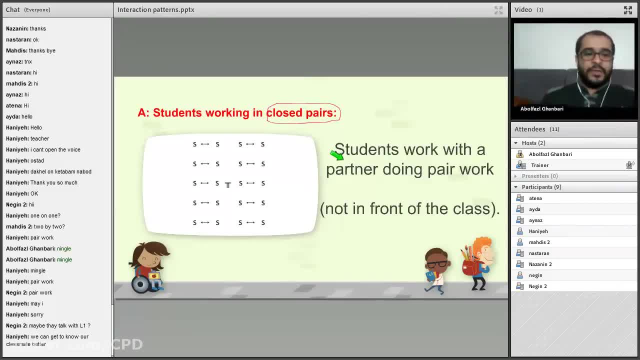 You can get to know all classmates better. It can be a good point. Yeah, So one of the advantages is that at the same time everyone is talking, So everyone uses this opportunity. But if you just want to do one pair, 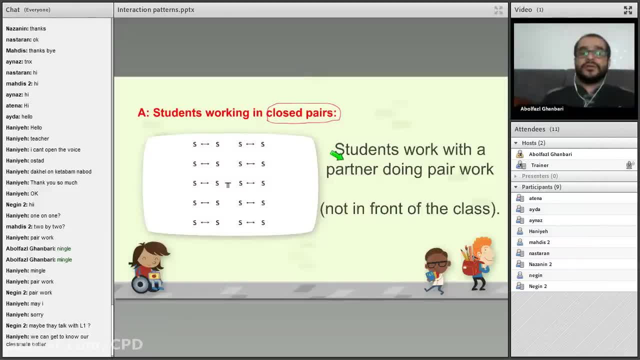 hey, did you see another teacher? He says: you two, the rest are silent. You two, the rest are silent. Then it's over You two. So what happens? One day? your class went bad and many of them haven't talked yet. 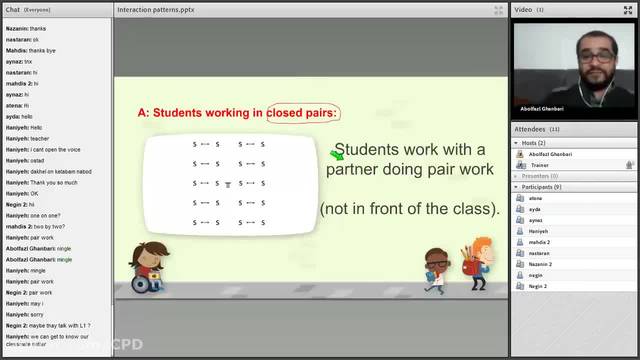 This is one advantage. Second advantage: Do you remember what we said in the first session? After two or three minutes, the attention of the students goes away. Now you have to tell them: Keep your attention here. Listen. He says I'm not with you. 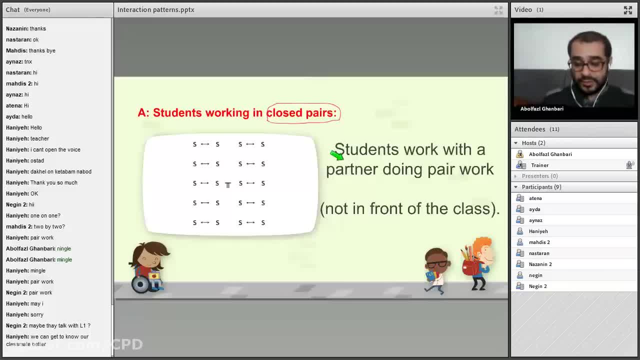 Pay attention, The students are talking to your friends. You can't distract the students anymore. This is another advantage. You two the rest are silent. Again, you two the rest are silent. But when we ask them to work in pair at the same time, 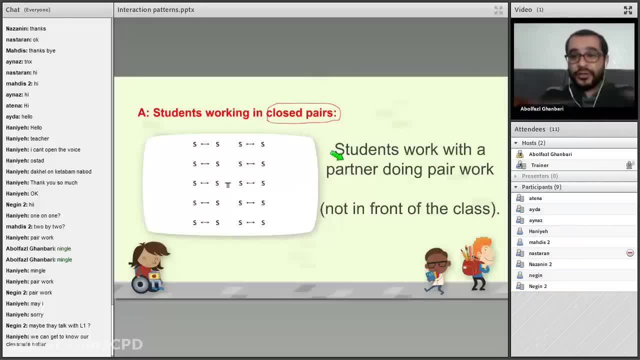 we contribute the time among the learners at the same level. They have the opportunity- It's called opportunity- for talking at that time And while speaking, while communication, while talking, while working in pair, the teacher monitors them. walk in the classroom. walks in the classroom, monitors them. 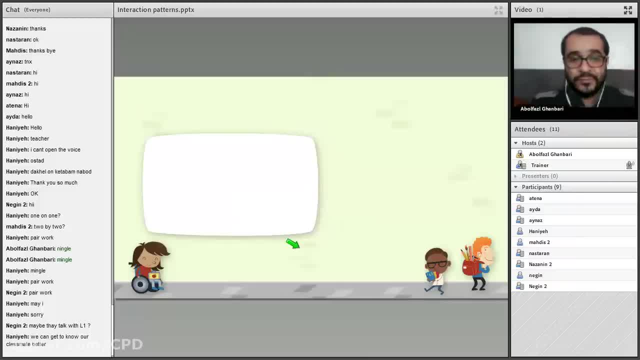 and write their mistakes. Yeah, Write their mistakes. This is close pair. What about this one? What about this one? Can you describe? what is the picture, what the picture says, What the picture shows? No, they are not open pairs. 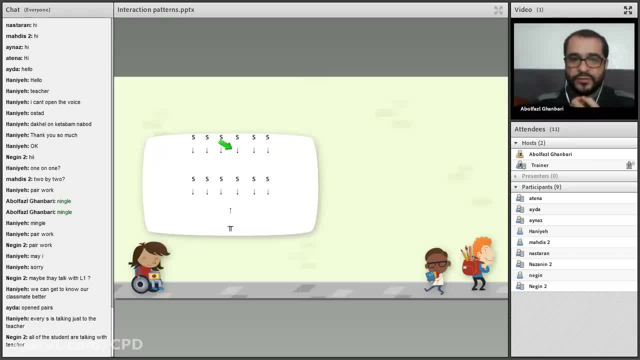 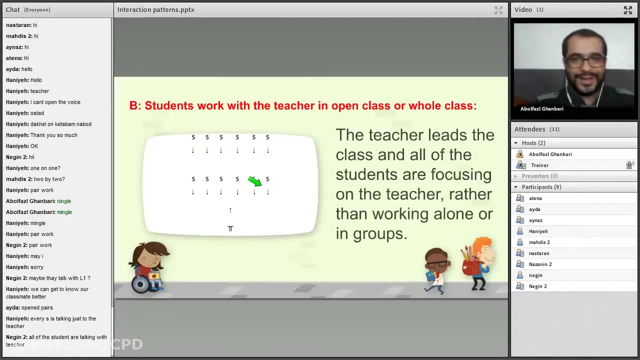 They are individual working. Yeah, The teacher is in front of the class And each student sits on his or her chair or sits And they are listening to the teacher. Yeah, Whole class or open class, The teacher just speaks in the classroom. 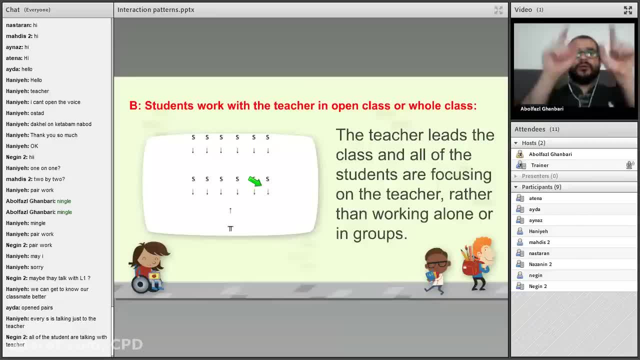 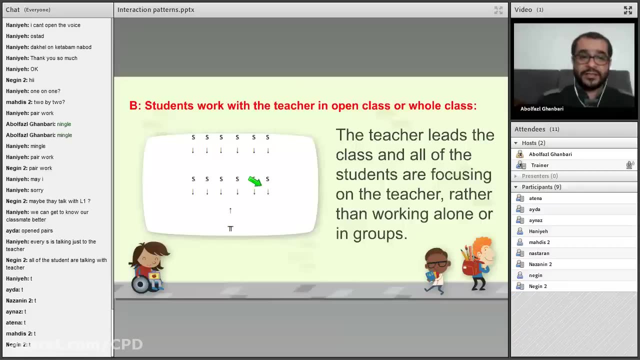 The teacher leads the class, Yeah, And the students are focusing on the teacher- Hello. Who talks more in this type of interaction pattern- Teacher or students? Teacher: Is it learner-centered or teacher-centered? Teacher, Teacher-centered- Teacher-centered. 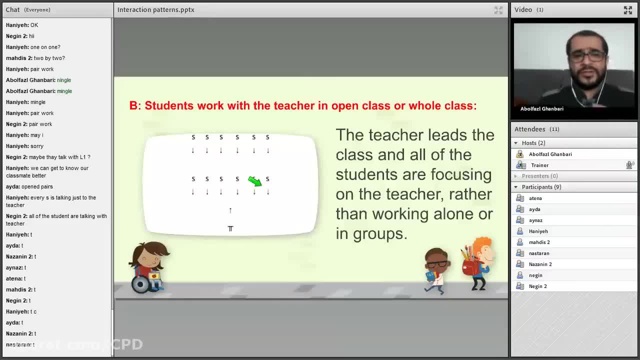 Teacher-centered, Teacher-centered, Teacher-centered, Teacher-centered, Teacher-centered. Hello, Hello, How may, how much time should be allowed allocated for this type of interaction pattern? How much time? It should be a lot, it should be a little. 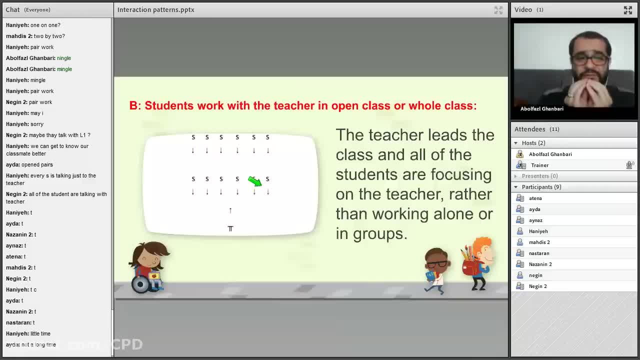 Yeah, It should be very, very a little time, little time, Hala. what is the disadvantage? or what are the disadvantages and what are the advantages, or what is the advantage? Teacher? the disadvantage is the students aren't active in the class and the 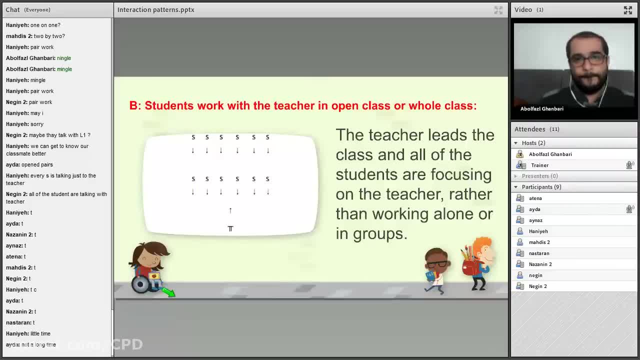 teacher: more speak. Yeah, the TTT is more teacher talking time and the student talking time at sun is not seen. It is one disadvantage. What else, Teacher? actually, I think this class is so boring, especially for me. It's so boring and because 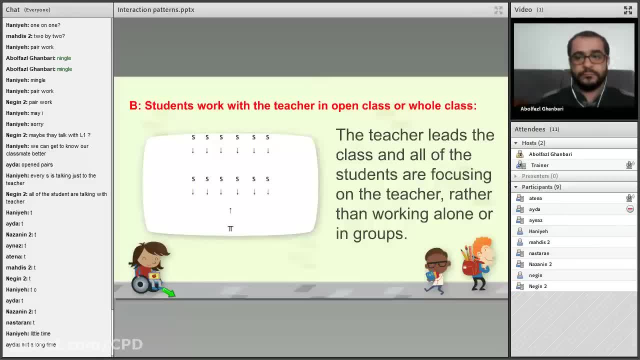 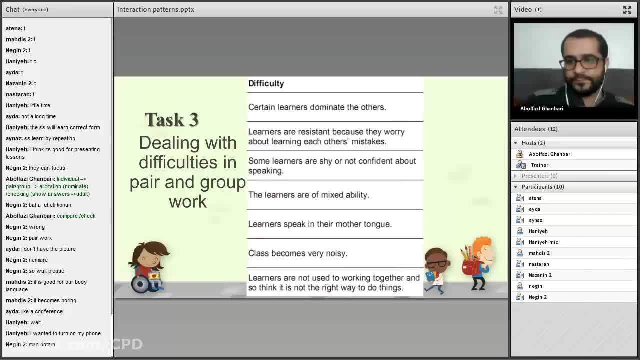 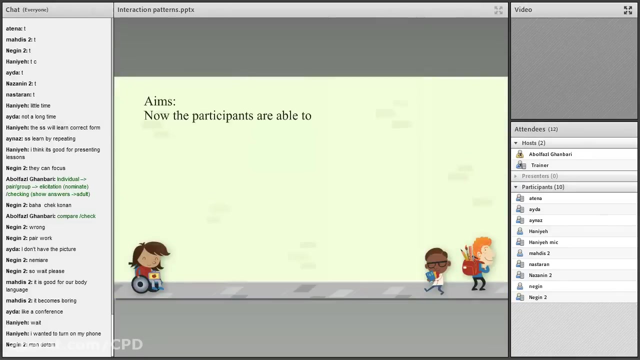 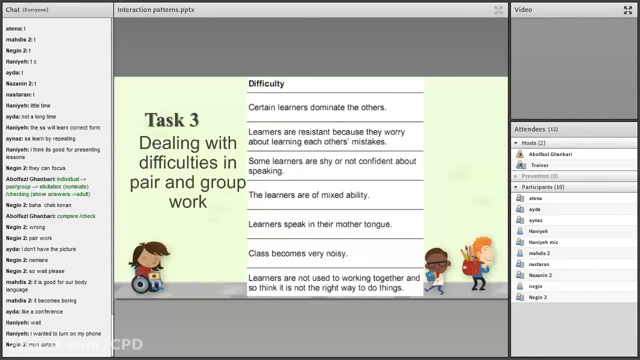 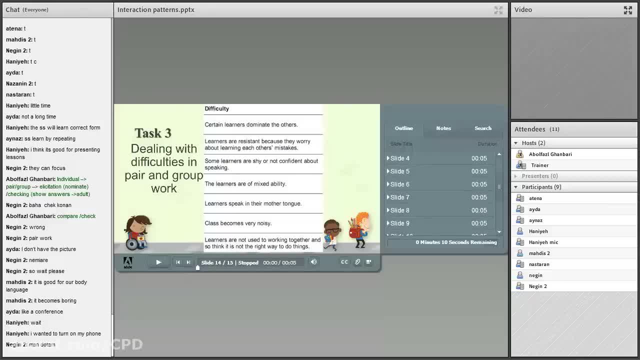 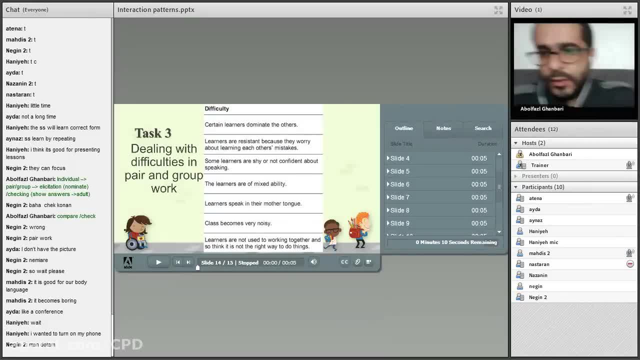 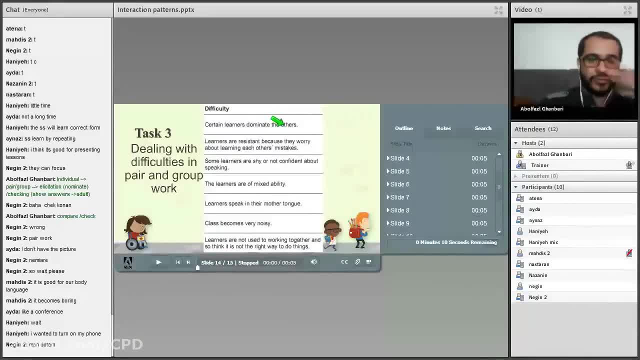 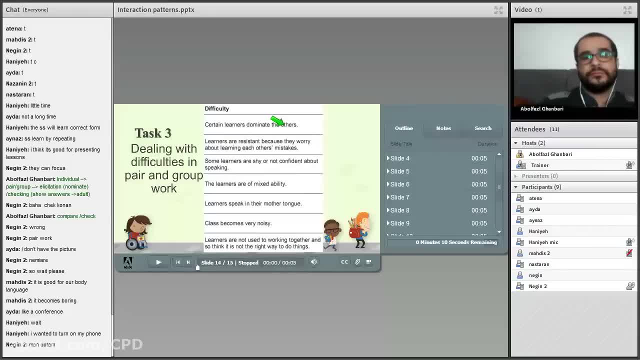 If we mix all of them in one group, all the groups will be divided. If all of them are in one group, then only one group will be active. Other groups will be active because of these dominators. If you want to go out, you can go to the other side. 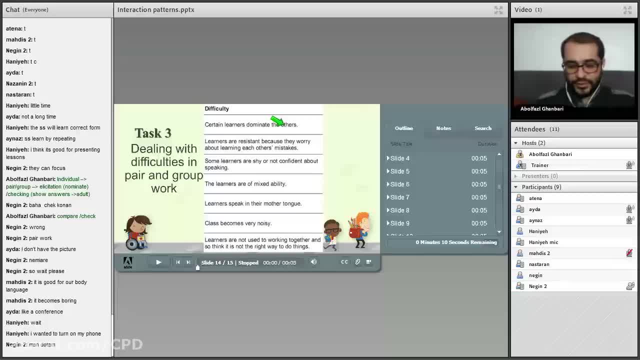 I will go to the other side. If there is really a group, then you can help the ones who are more dominant or have more power to talk. So one of the solutions is ask them to aid their participants. How you can ask them to aid their participants. 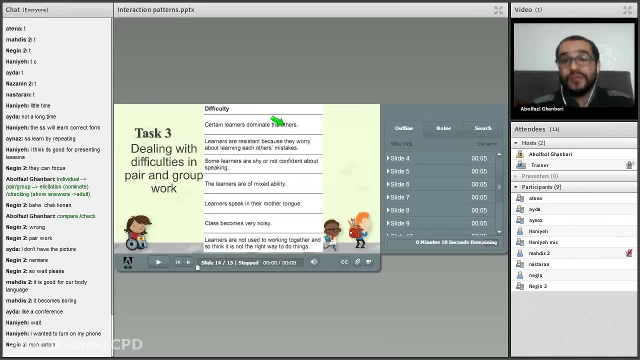 We should give responsibility to them. We should give responsibility to them. We say, for example, you are the leader of this group and you are responsible for helping the students to reach this level. Right, You can ask them to do the same. 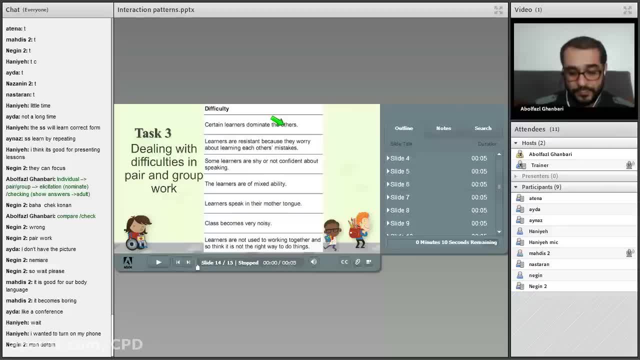 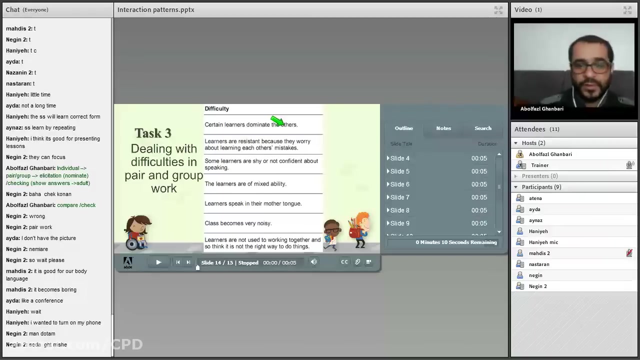 Ask them to do the same. Say it, Say it. If you give them a responsibility, they can decide that their level is good. If you help them to do some things, they will be positive. Learners are resistant. they don't want to work with others. 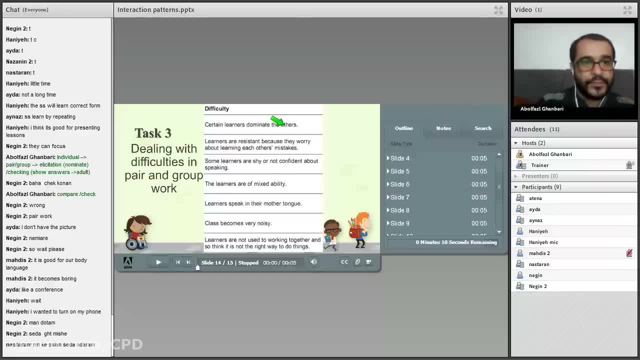 What should they do? You will need to ever exceed those fears of making mistakes and tell them that if you make a mistake or if you understand something wrong, you will make a mistake and you will make your mistake correct. Just in order to understand what you think about this topic, you can share your idea. 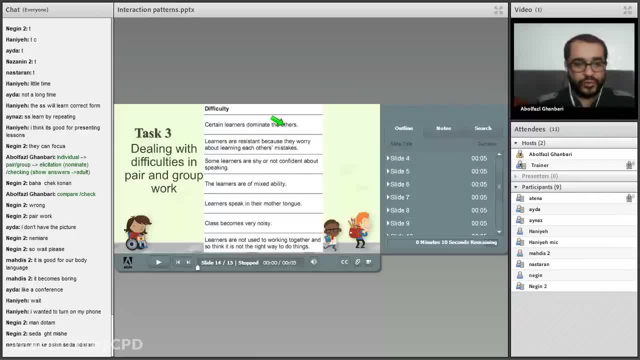 Thank you, It was a very interesting talk. I don't have a voice. What do you mean? I don't have a voice. Do you think everyone has a voice? If you don't have a voice, write down the number 2.. 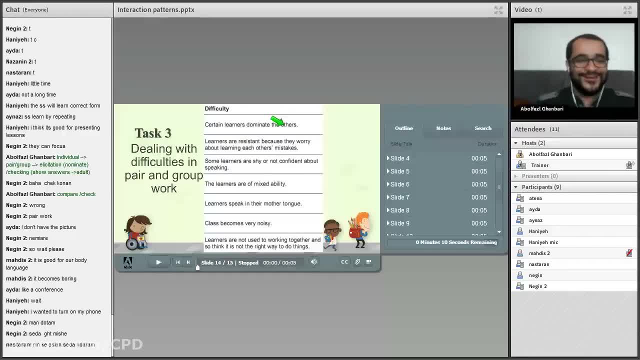 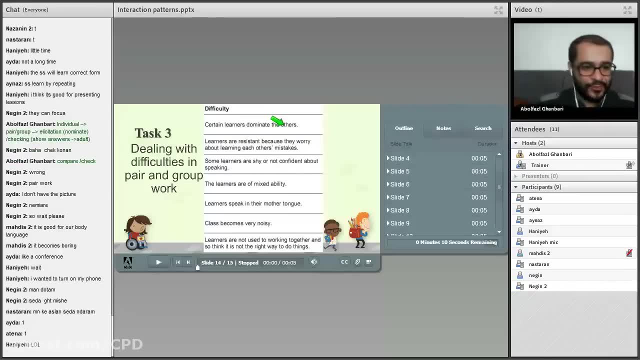 If you don't have a voice, write down the number 2.. If you have a voice, write down the number 1.. Let's say everyone has a voice. My internet is full. Do you have ID? Do you have ID? 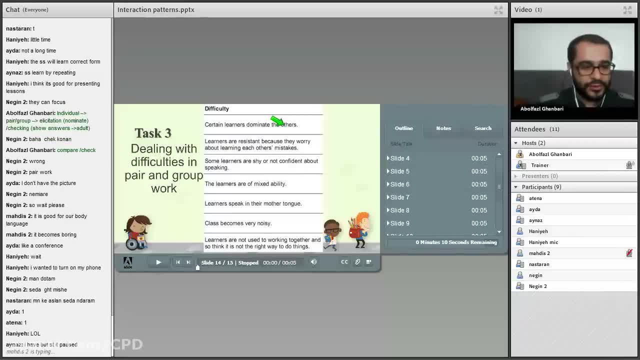 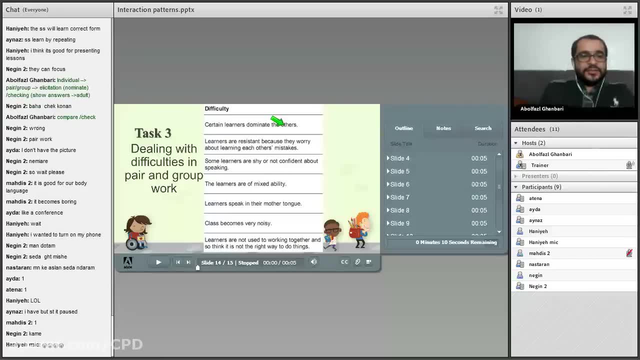 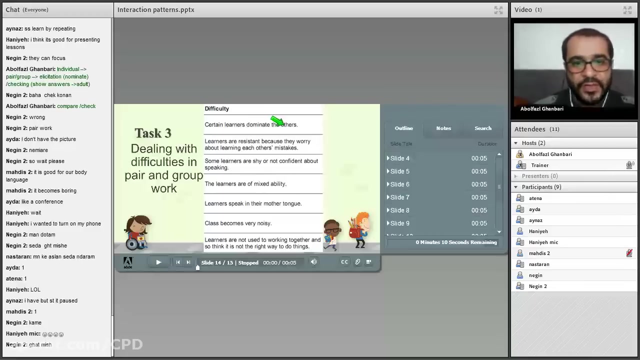 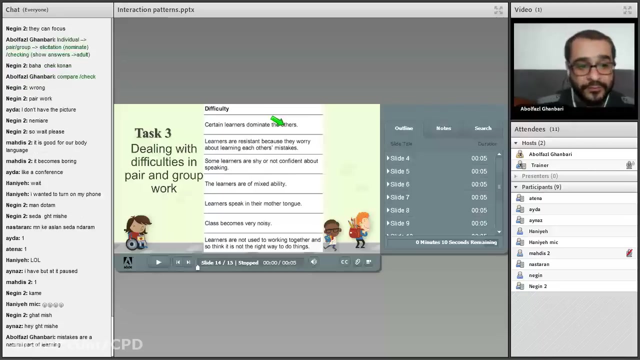 I have what. It is paused. What does it mean? It means that someone is using your internet. If someone is using your internet, you will face problems. Yes, someone is using your internet. We should explain the learners that mistakes are a natural part of learning. 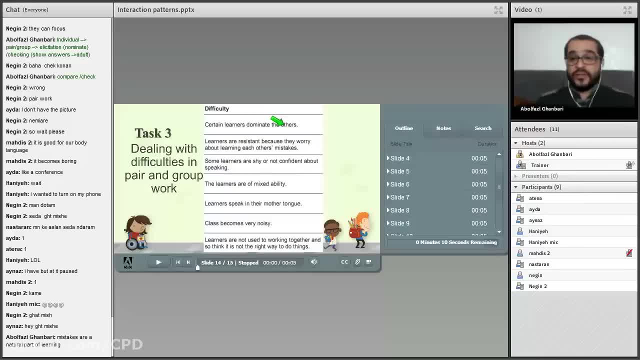 I mean without mistakes we do not learn. We should listen to find others' mistakes. This is one part of our learning procedure. The learners need to know. If you do not encounter mistakes- other students' mistakes- and you do not recognize their mistakes, you do not learn. 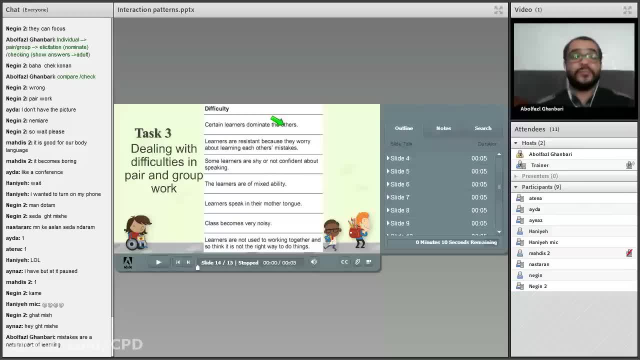 And because of that, we need to work in pair, work in group? Yes, And this is a natural procedure of learning. And again, again, by monitoring them, by monitoring them, and, as a teacher, we walk in the classroom. 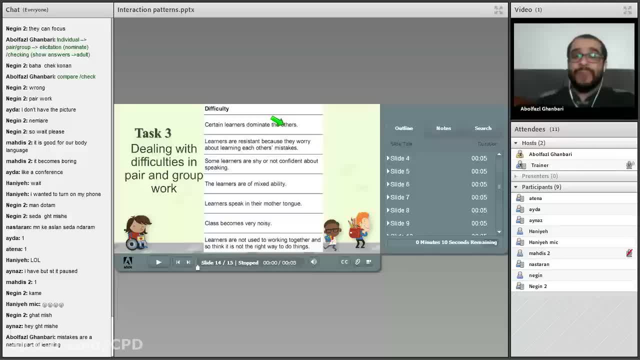 we monitor them, we make sure that we make the learners sure that, yes, we are monitoring and we aid you. we help you to learn, we aid you to find the mistakes. Yes, These are two important solutions for this mistake, this problem. 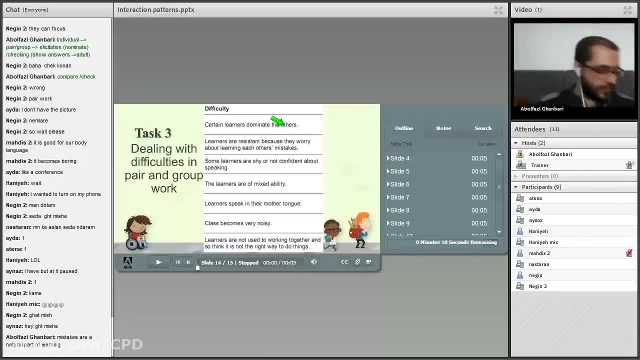 The next one. some learners are shy or not confident about speaking. Yes, And the sensor is the most important. You should praise them to talk, for example. when they talk, You should say: that was really great, You come below and talk. 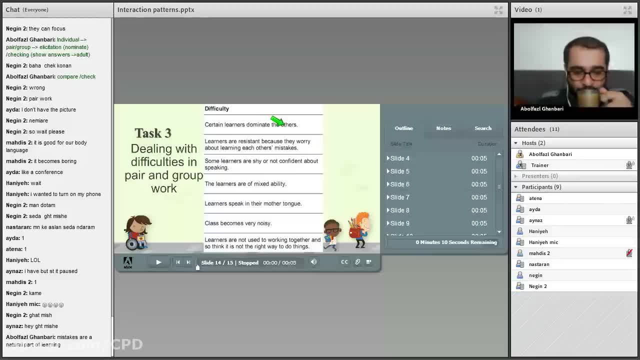 Okay, Okay, Can you hear me now? We should praise them to talk, for example when they finish their speaking. After that we should say: wow, that was great. And we should stop bullying at him or her, And, for example, when other students laugh at her. 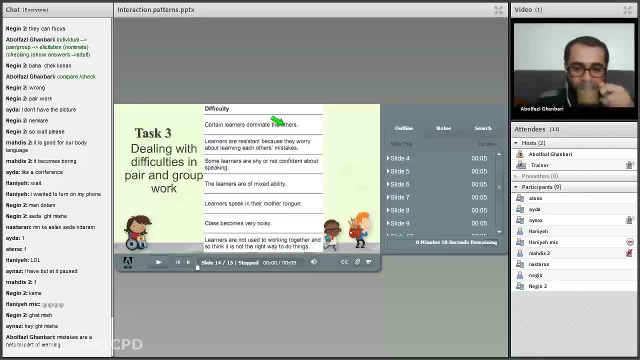 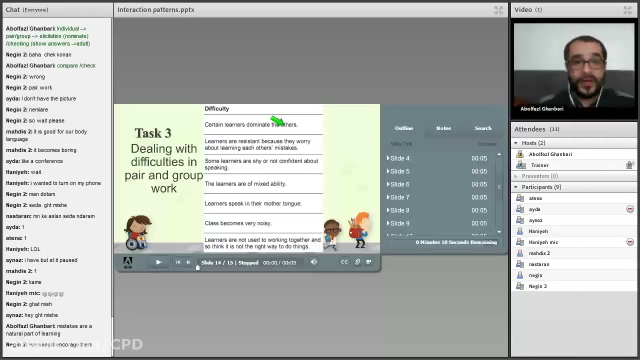 we should, for example, say that our students do not do it again. Very good, It works, Very good. Praising talking to other students not to say something. Do not correct them repetitively. Yes, encourage them. 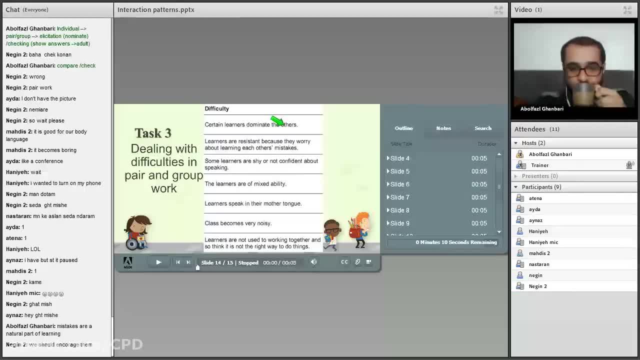 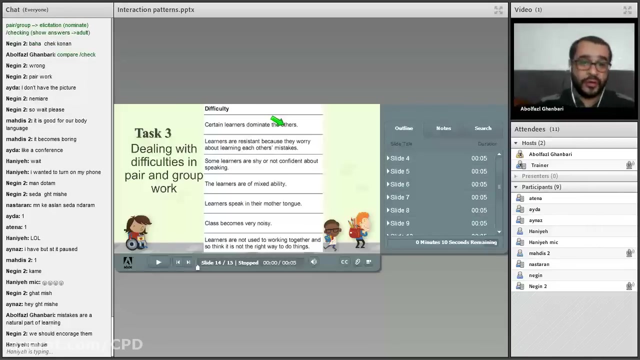 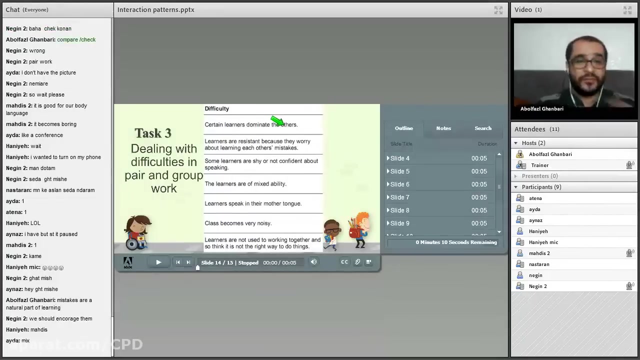 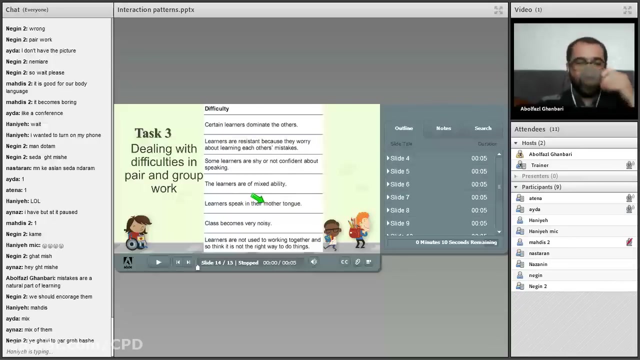 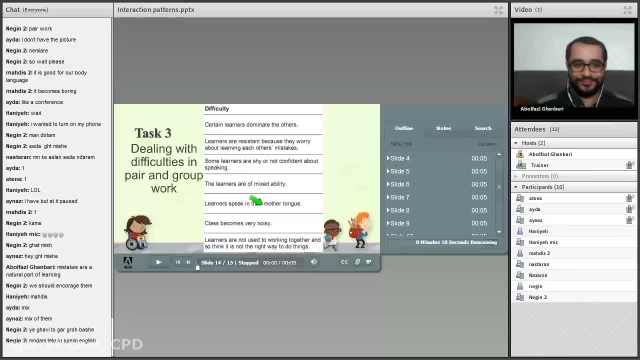 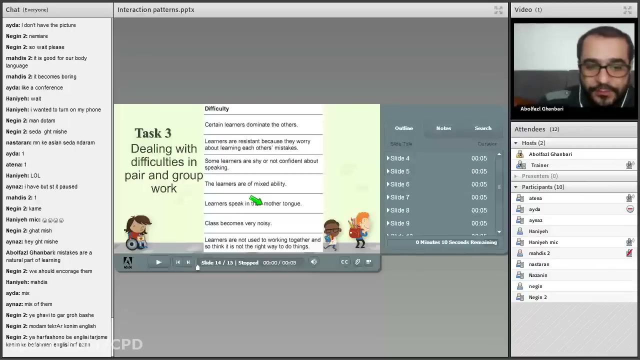 You can speak English with your friends and family. When a student speaks Farsi, we repeat the same sentence in English. We say: يومينتس نگيم said that we should translate the words so they can understand when they speak French. 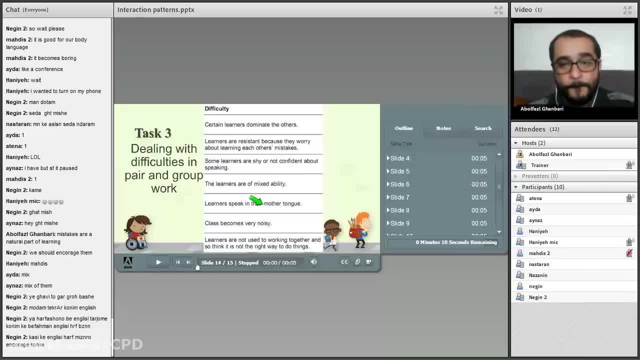 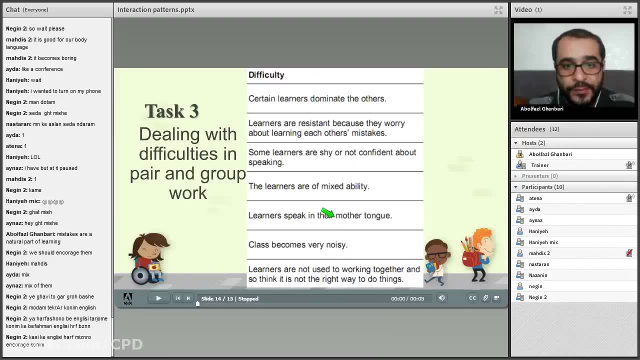 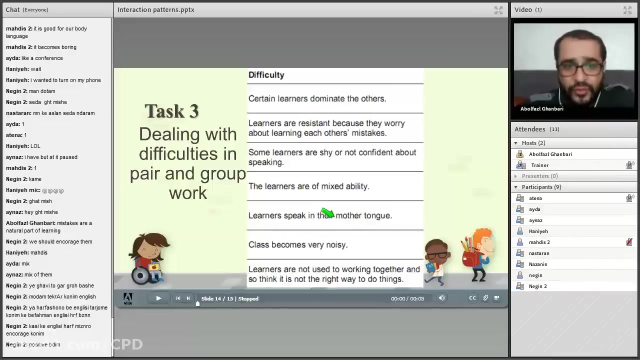 That's what I think, Because a lot of teachers, when we speak Farsi, they repeat the same sentence. First of all, let's see why they speak Persian. Yes, it will be helpful, But how? First of all, let's find out why they speak Persian. 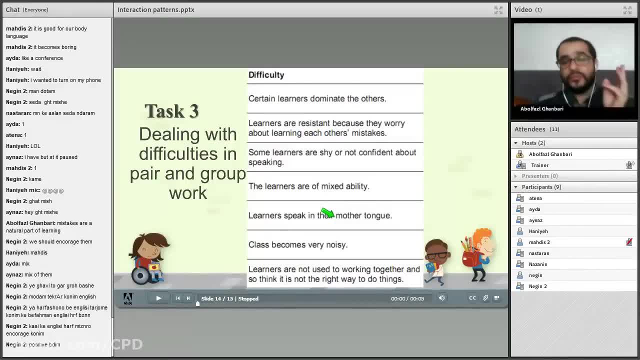 First, they are teaching something. They want something that is more than their level. More than their level. This is one of the reasons. So let's see what we want. Is it more than their level or not? It's not important that the book is, for example, a book. we say, yes, the book is a passage, but these children can speak Persian. 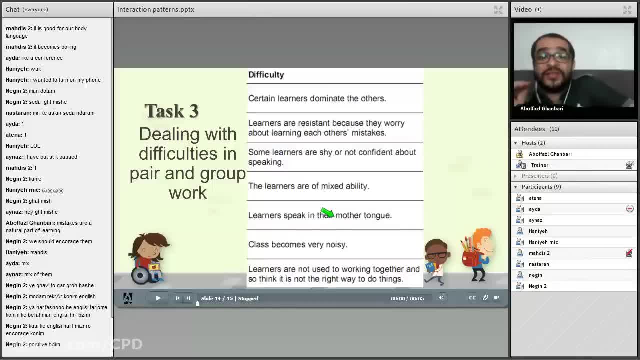 No, this is not important. It's important to see the level of the children. If the level of the children is low, then we have to bring down our activities and our desires. It doesn't matter what books they read. We have to bring down the points so that we can help the children to come up slowly. 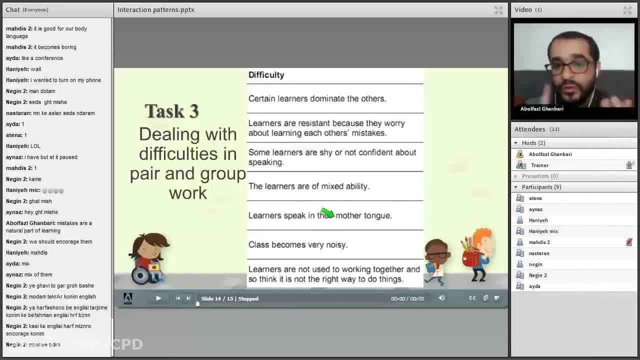 This is one point. Second, the sentences they need to speak are not valid. What sentences do they need to speak? Classroom languages. So let's teach them classroom languages. We remember, I told you classroom languages. We will teach you how to use them and how to use them. 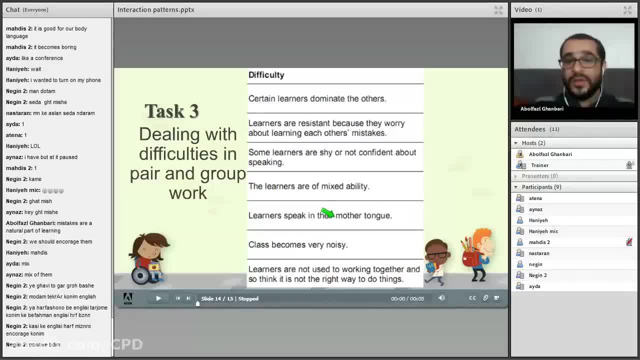 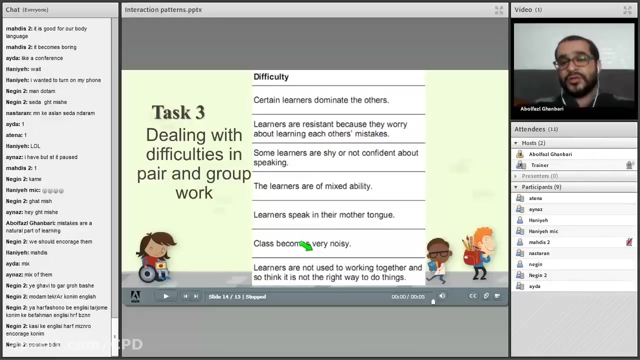 Is that right? Then, if they switch to L1, remember them. What could we say in English? Remember them. This will happen for a while. Well, Class becomes very noisy. Class becomes very noisy. Class becomes very noisy. You see, we have a noise that's ordinary. 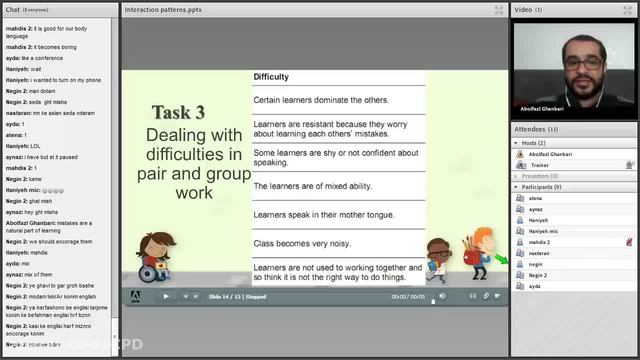 When these kids are doing thelands well, they speak normally And we don't have to say why this noise exists. But there comes a time when the noise is very noisy. There can be a lot of noise. Hey, Hey, Hey. 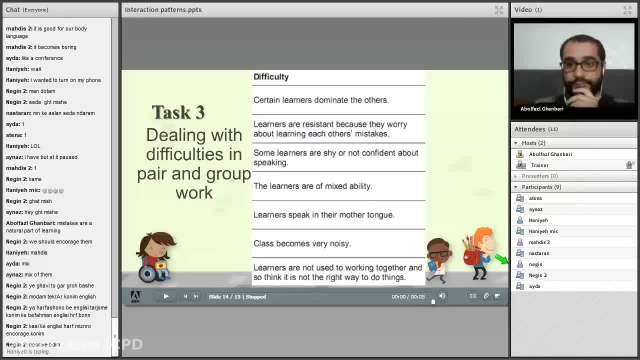 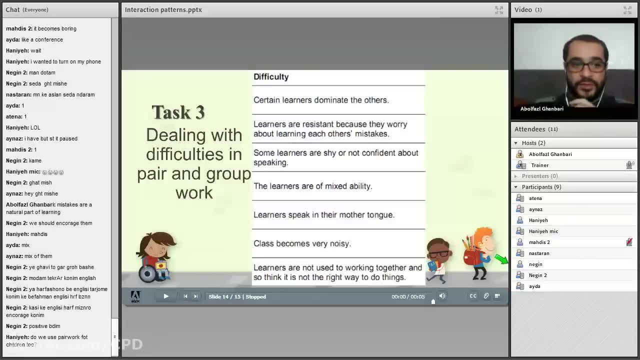 Thank you, Say it. Say it in positive or negative. Yes, children should have the same power group. I don't have any questions. I said I think we can give them some activities that, for example, I don't know- play songs or paint movies, or we can learn them and teach them that to. if they have or they want to say something, raise their hands. 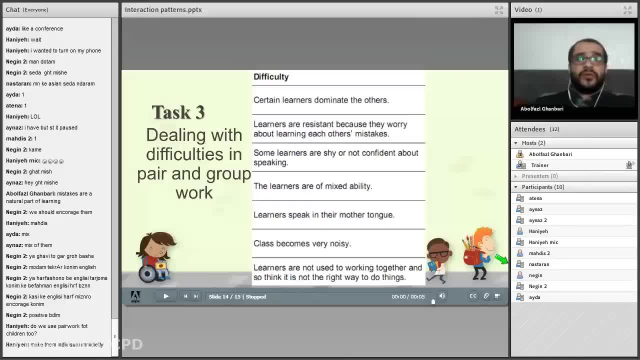 Well, this is a time when we are supposed to have whole class activities. But we want to have a whole class activity, That is, the children should talk to each other in that way. We can't say, for example, everyone be quiet, just you two talk. 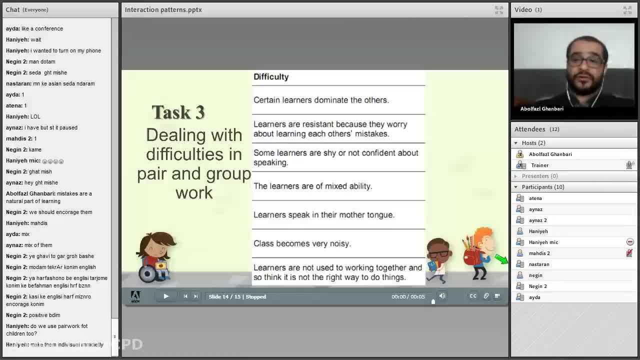 They should practice, Because these are exercises. you see, these are not tests, these are practices. When the children are in the middle of the class, they should have the opportunity to practice. That's right. We now have 50 minutes of time. 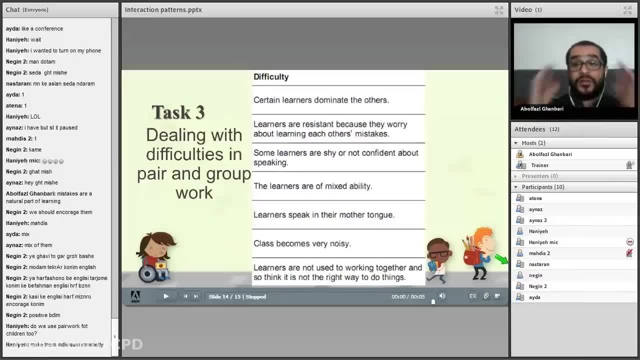 I have to practice for 50 minutes to learn. I can't just practice for 5 minutes in 50 minutes and the rest of them sit quietly like this. I can't sit either. Neither does my learning style and learning characteristics allow me to do this. 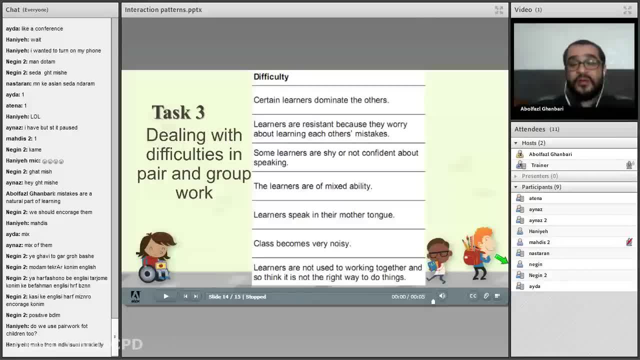 And neither does the class. It should be like this: I practice for 5 minutes and the rest of them don't practice. So I practice all the time. So we can't say, for example, just you two talk and the rest of them listen. 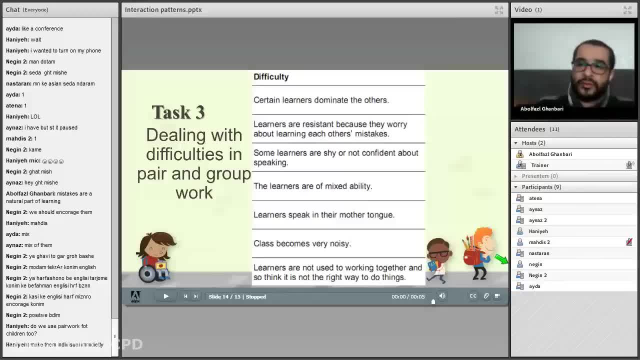 Well, it's over now. you two talk and the rest of them listen again. That's not how it works. We have to at the same time, all the learners talk, All the learners working pairs or working groups, So it's fun to be quiet. 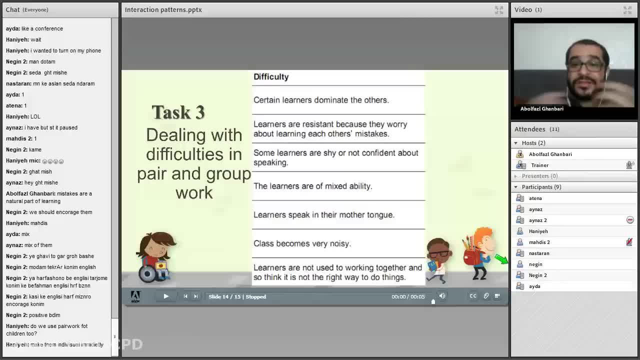 We have to, as we say in class management, we have to define the rules for the class. We define the rules When we see that the noise of the class is going up with one attention, for example, clapping. We practice clapping with the children. 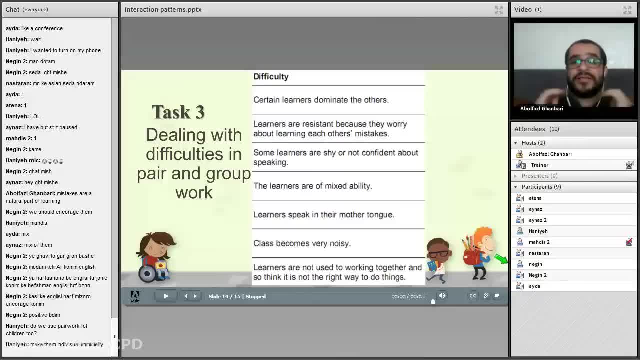 In the first year. they say, for example, when I clap, the noise increases, Practice a little slower. That is, they clap slower. You see, some of them clap like this, They clap like this. We want that pair worker. 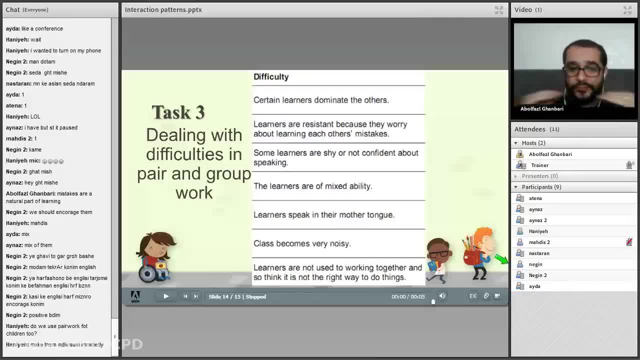 It must be, But the sound is normal Lower level. We practice this with the children. We practice this with the children When they hear this attention, that is, the level of the sound goes up. The level of the sound must be at the bottom. 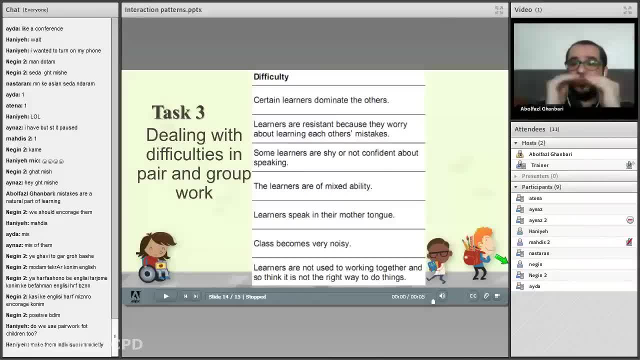 But the sound must be normal. We can't just say that there is no sound. If there is no sound, then there is no practice, And if there is no practice, then the class is not going to work. We share this with you. 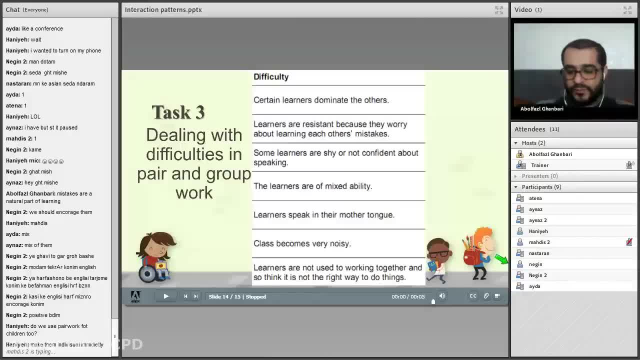 I share this PDF with you so that you can read it. There are different ideas. We share this with you so that you can use it in your class. Well, no, we don't take it on the individual, Because they have to do pair work. 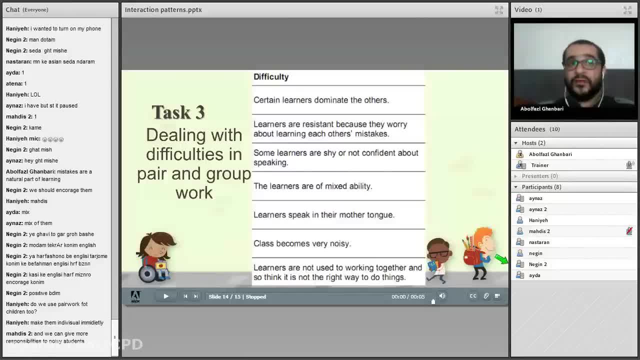 In fact, the class doesn't care if there is no pair work or group work. What makes the class, more than anything else, Pair work and group work- If your class is 90 minutes? Well, if, for example, it is 90 minutes, 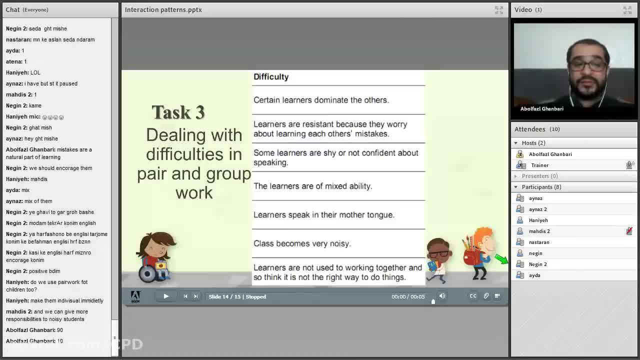 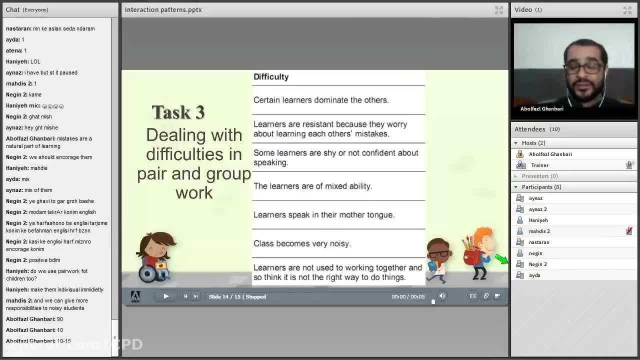 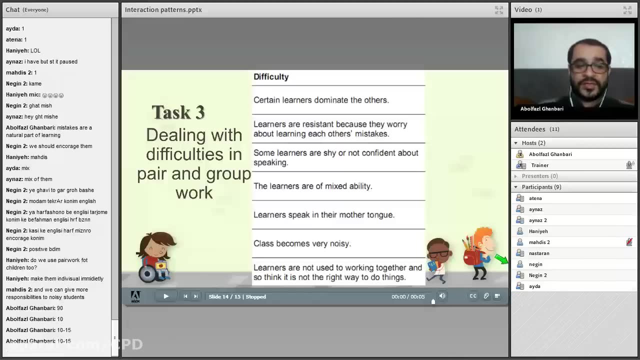 The teacher does not speak more than 10 minutes. 10 to 15 minutes. What about the rest? The rest is pair work, group work, individual work. What about individual work? It is also 10 to 15 minutes. The rest, for example, now it is 30 minutes. 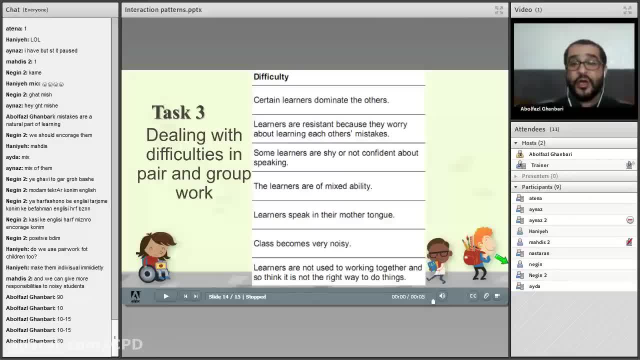 The rest is 60 minutes. The rest is 60 minutes. You have to do all of them: Pair work, group work, pair work, group work. It is not a standard class. Why? Because I don't have time to practice in that class. 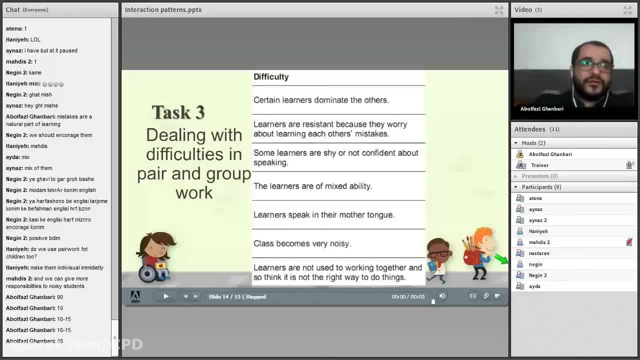 I always have 5 minutes to talk in that class. Do I learn speaking with 5 minutes? No, In a 90-minute class I can talk for at least 60 minutes. 60 minutes I have the opportunity to talk. 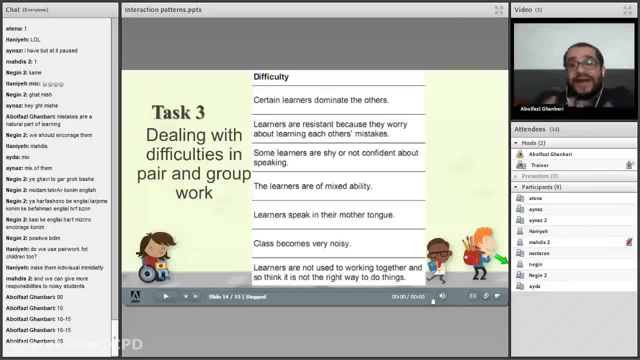 How is this possible If I only talk for 60 minutes? what about the rest? We have to have a pair work, group work. What about the rest? All of them have the opportunity to practice speaking. At the same time, all of them have the opportunity to practice speaking. 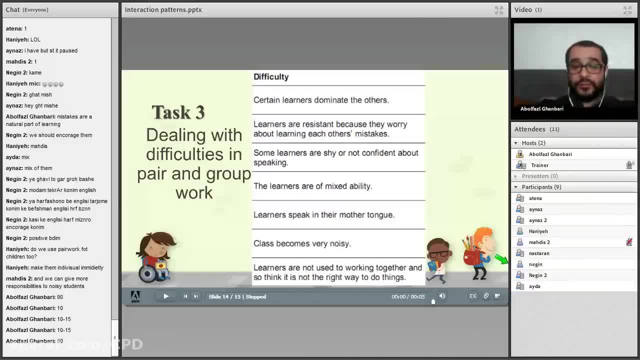 When I say, guys, you saw, I gave group work. In this group work, you all talked to each other. Well, some may not have talked because of the internet connection and microphone problem, But in that 5 minutes all of you had the opportunity to see your eyes. 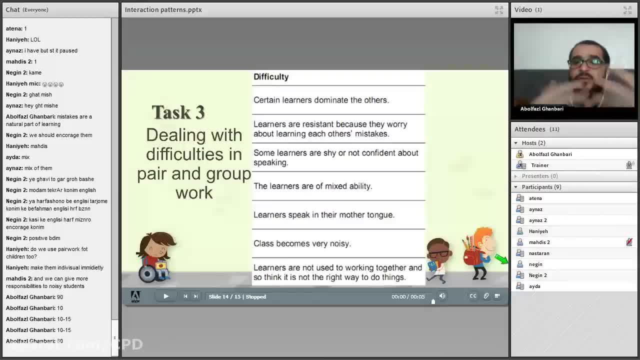 Now, if this time is more, you will also have more time to talk to each other. Our class, our base activities, should always have pay work and group work in it. Your class should be online and your class should be present. The most time of the class should be pay work and group work. 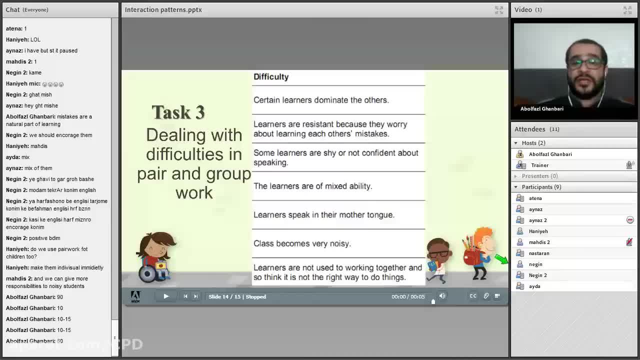 If you went to a class and saw that the teacher was talking, the teacher's talking time increased. That class does not hurt. Neither you go to that class, nor do you recommend others to go to that class. That class does not hurt. 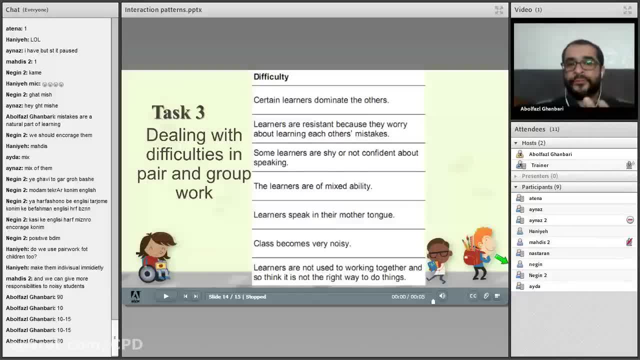 2. If you went to a class, the teacher does not talk, but the children work individually. If someone wants to talk to a woman, let him do it. It is individual. Again, that class does not hurt. No one there learns speaking. 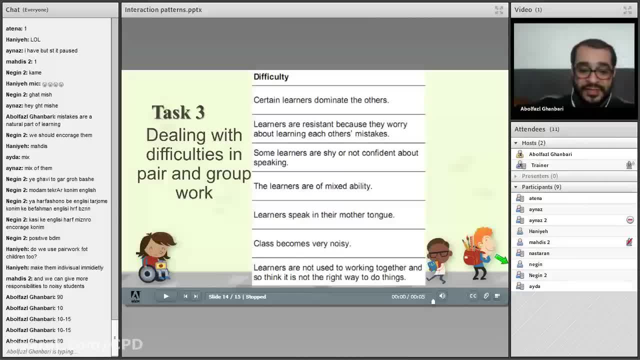 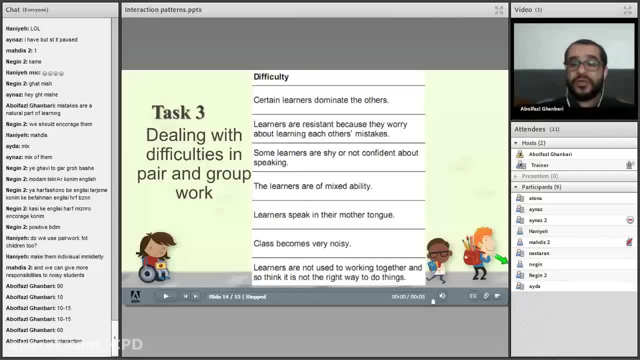 He does not learn the language. We learn the language in time. We do not learn the language. We have to have interaction, Interaction. No one learns the language without interaction. We will talk about this later. What else If you went to a class? the children do not have pay work and group work. 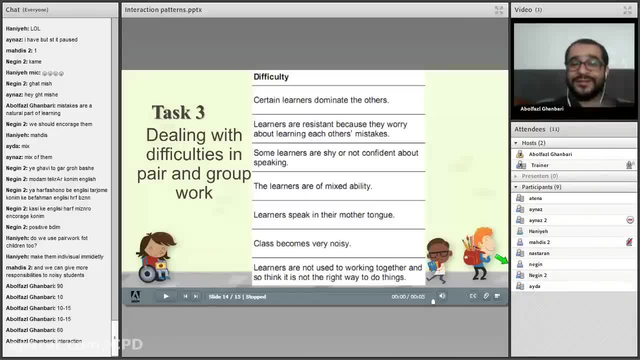 Again, that class does not hurt. The children talk, but how do they talk Internally? Well, you speak, Only you speak. You speak, Or they only speak individually, Or these are open pairs. What was Opening pair meaning only 2 people are needed. 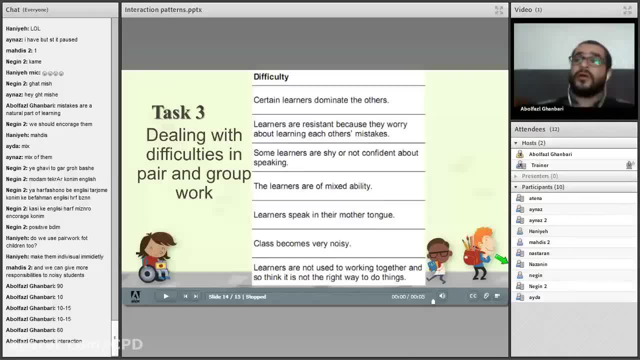 Just two, 1500 people And expect to speak the other person and get to talk. Why, Infact, lt is not a problem And these lessons are not an issue. No learning, And you should take part in this lessons. If I want to be a teacher, I have to give input, give instructions, go to paywall group board and I monitor to see what the students are doing. 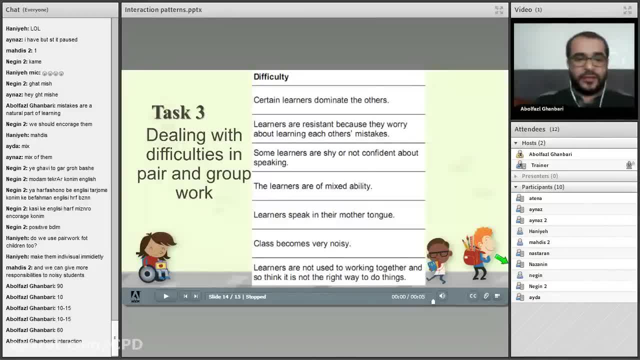 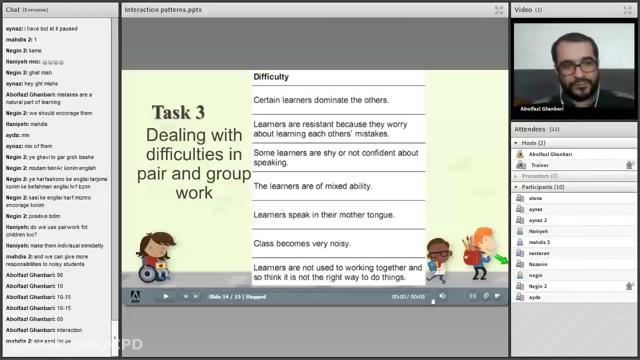 That friend who recorded my grammar session. why didn't you put it in something? You didn't put it in the group let the students see it. You left it in our group. but because the internet is very weak, your voice doesn't come in the video at all. 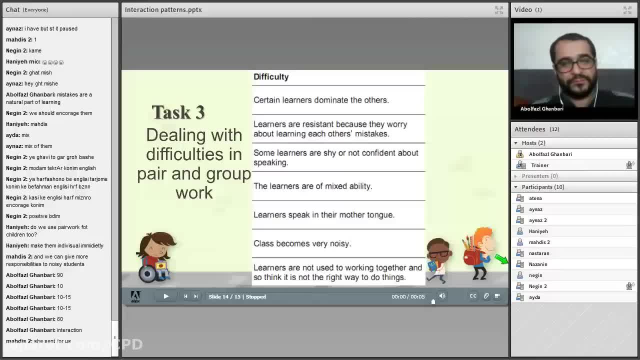 Because I said that I wish you would leave it in the video. It's not possible to leave it in the video. It was three times. I left it in the video. I don't have anything to do with it. It's not possible to leave it in the video. I don't have anything to do with it. 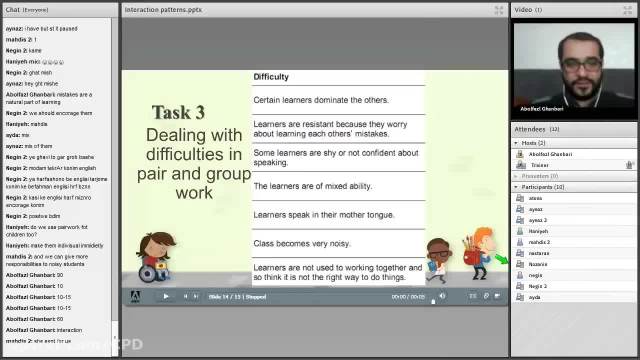 Well, this is the end of this session. Now you are able to study different types of interaction patterns, to come up with their advantages and disadvantages and how to treat different problems. may we encounter? Thank you, We will encounter in the class soon because of using different types of interaction patterns. 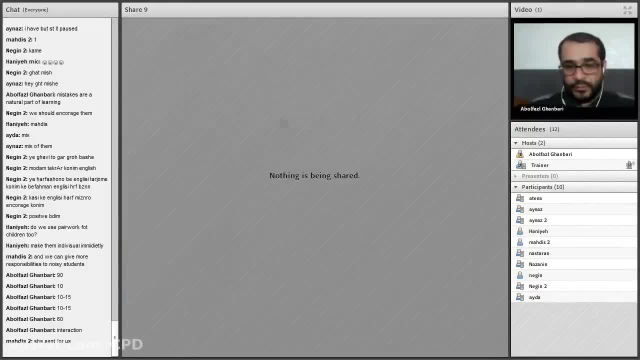 Well, this is the end of the session. 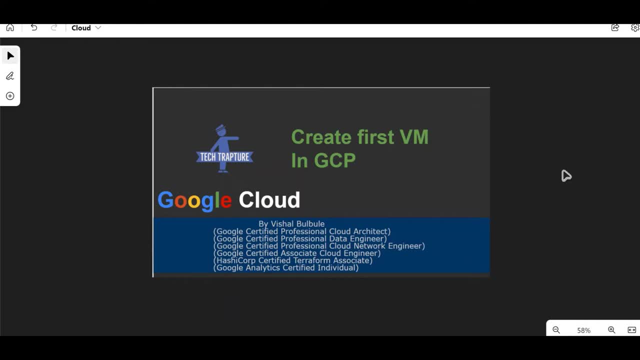 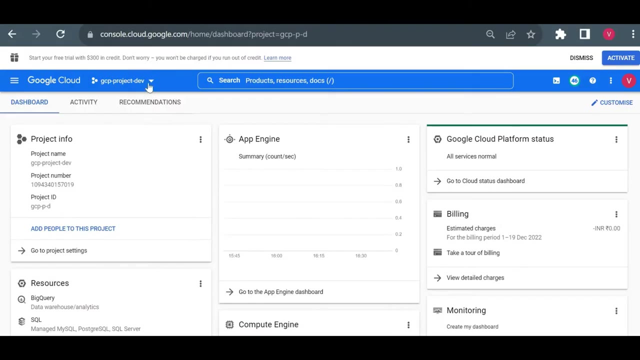 hello all. welcome to tech capture myself, Vishal Bulbul, and in this video we are going to see how we can create our first GCP virtual machine, or we also call it as a GCE instance, that is, a Google Compute Engine instance. so first I'll go to my Google Cloud console. so I assume you already. 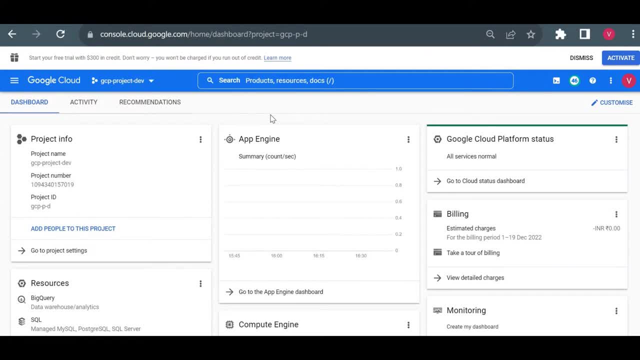 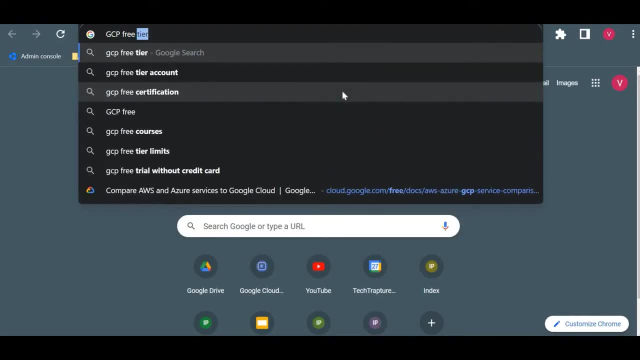 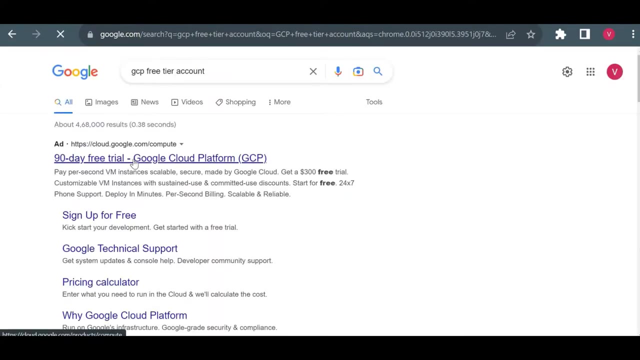 have your Google Cloud account. if not, you can create your free trial account. so I'll just show you how we can create a free trial account. you can simply type a GCP free tier account and you will see this 90-day free trial. so you can click on this. try Google Cloud for a free. 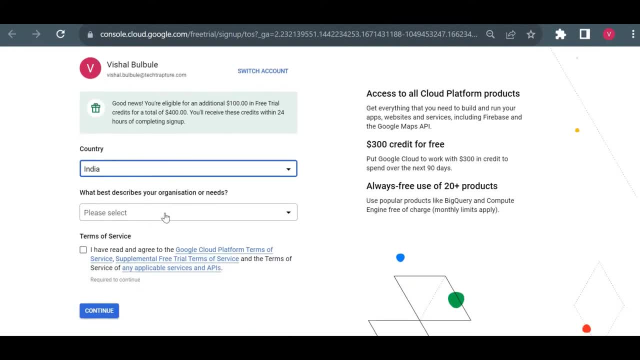 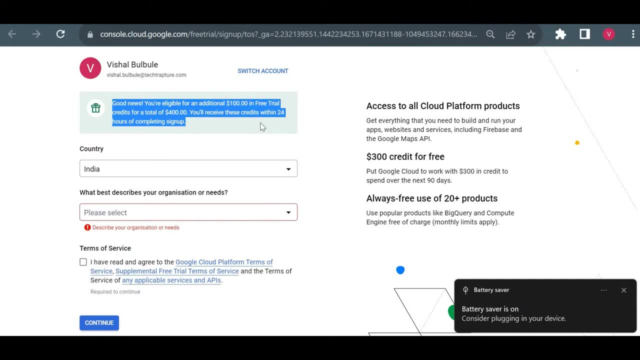 okay, so here it will ask you for details. we have to choose your country and now you could see- uh, this is a good news- that credits. earlier this credit was 300, now it's increased to 400.. so you will receive this credit within 24 hours of a completion setup. so that's just a suggestion. 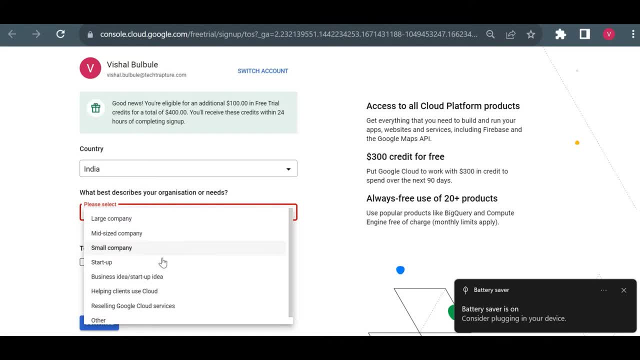 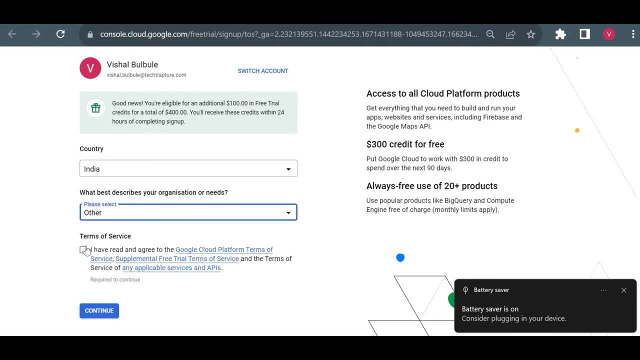 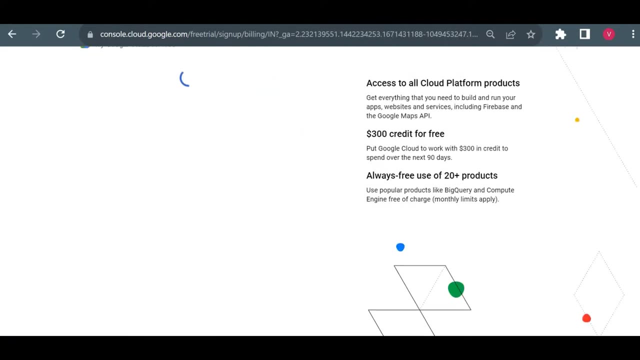 they are mentioning for you kind of offer and you can just uh mention here if it is your startup or what kind of. you can simply put others and you can click on continue and you have to mention your credit card details here. they won't charge you, they will just charge. 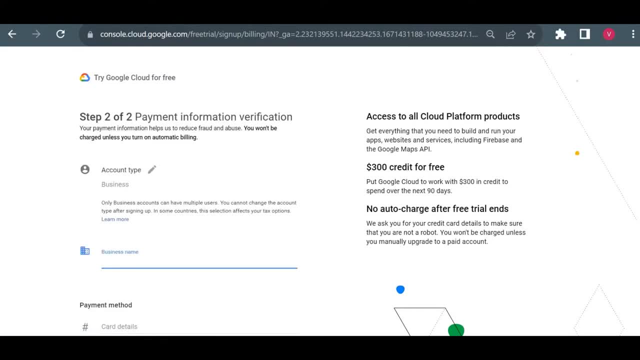 you, uh, two rupees. so here you have to mention your business name and your card details. so once you put a card detail, they will send you one time password to your mobile and you have to enter your one-time password and they will just charge you two rupees for a confirmation and they 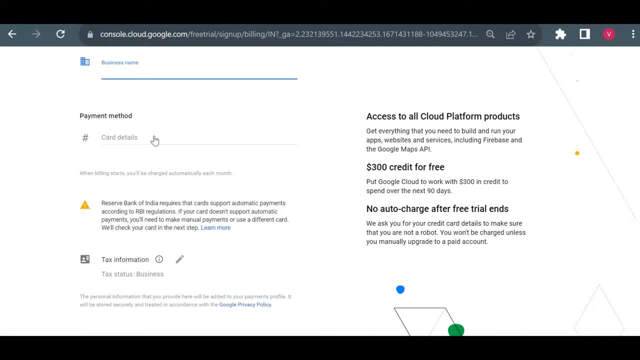 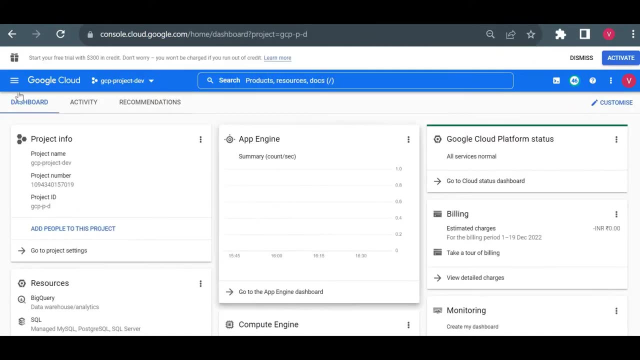 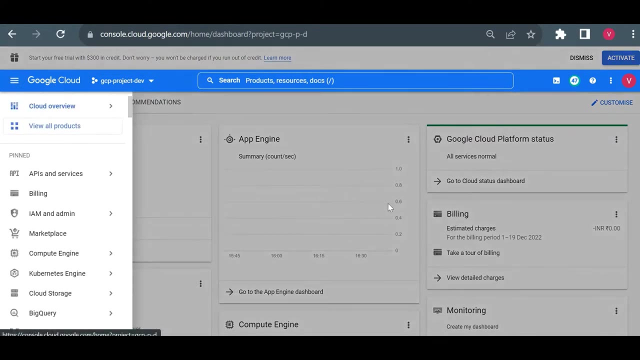 will just credit back a couple updates. so that's the process for creating a free trial account. so now i'll go back again to a virtual machine page here. so in cloud console to create a virtual machine you can go to this menu, navigation menu, and from here you can click on compute engine.